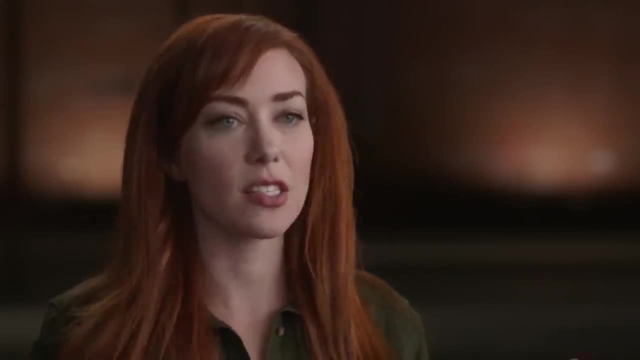 view, which is the whole reason why you go to a stadium other than the hot dogs, you have to design such that you know where the forces are going and how to direct them. the university of fayetteville is one of the largest stadiums in the world and it's the largest stadium in the 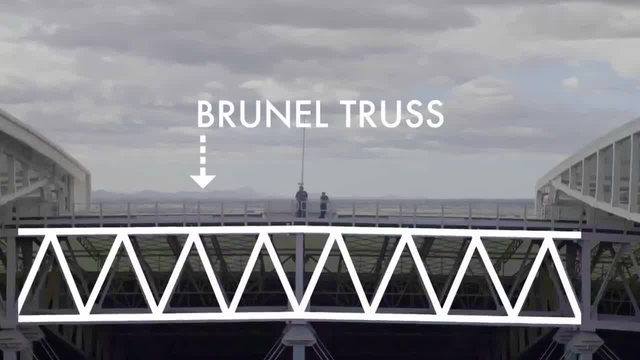 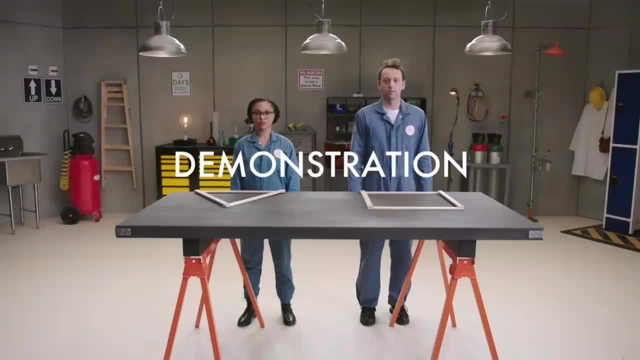 phoenix stadium actually employs brunel trusses. this is a kind of structure that really supports the stadium's roof using an arch that's formed a lot of triangles to bear the load. let's examine the strength of triangles. rectangles, when subjected to force, easily collapse into rhombuses. 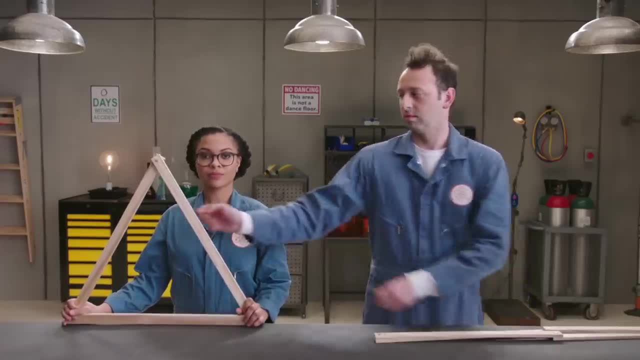 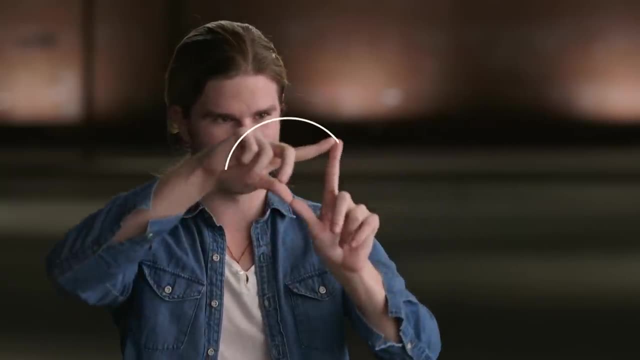 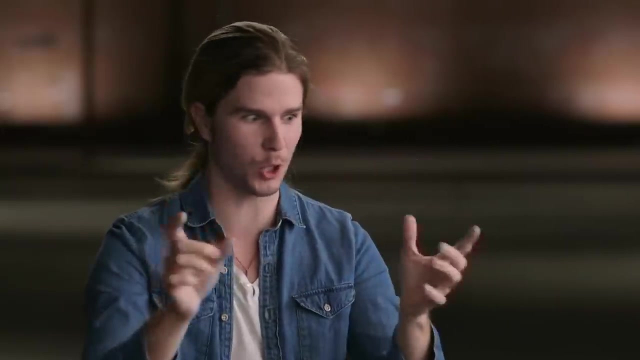 but a triangle distributes force down its sides and maintains its shape. so take this triangle and start tilting it and trace where the tip is and what shape does it make? an arch. so the strongest point of an arch is almost every point along its curve. and if you want to support 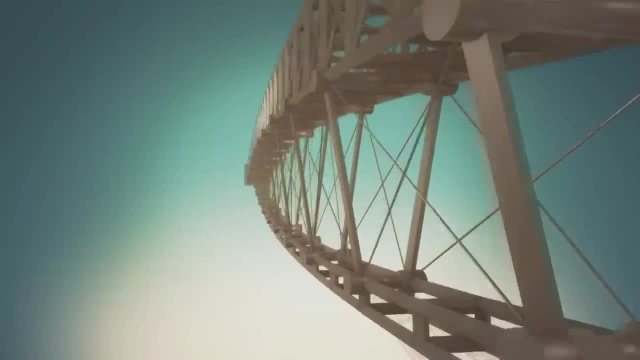 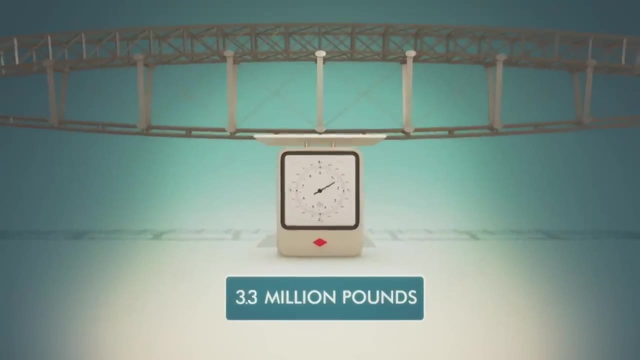 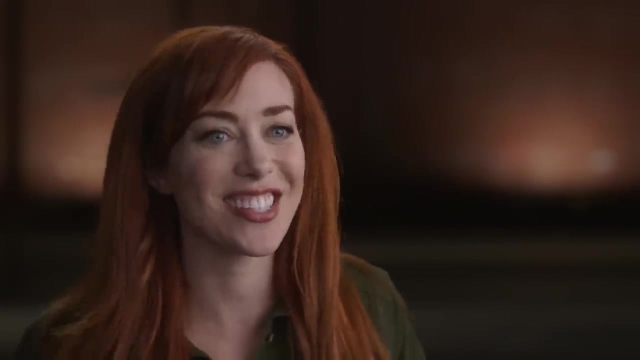 that. just add more triangles. your trusses will be made of solid steel. each will measure 700 feet long, 87 feet high and 17 feet wide and weigh 3.6 million pounds. i can't even fathom how many donuts that is. everything is measured to me in donuts, so it's a lot of donuts. 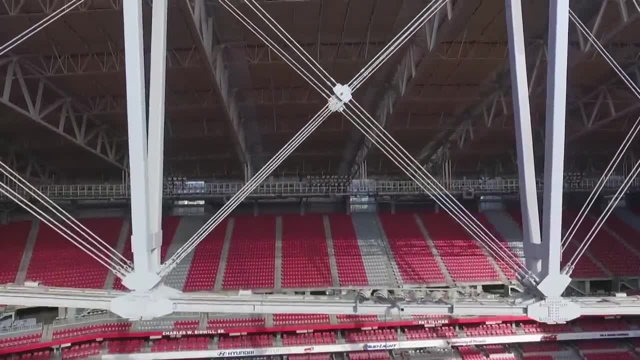 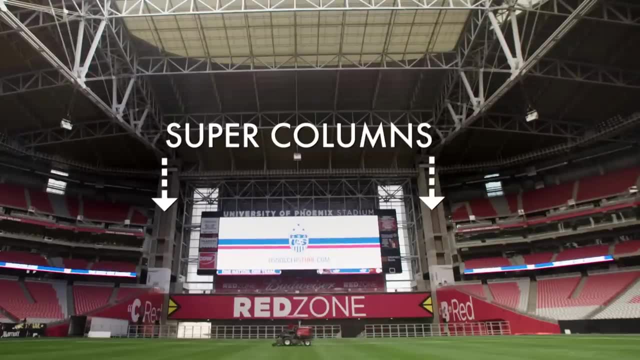 after constructing and connecting both of your trusses on the ground in start to finish the construction of the trusses, you'll need to make sure that they're installed on four 171 foot tall, 17.5 foot wide super columns. now you have a roof support. 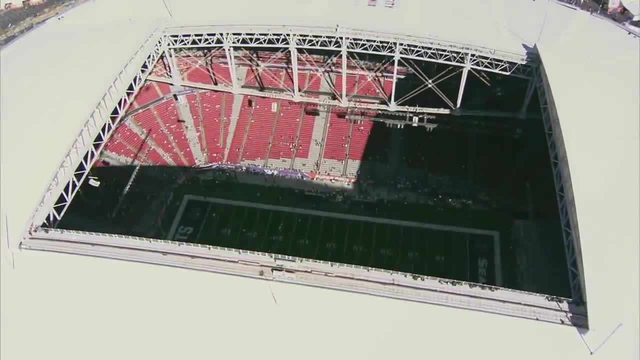 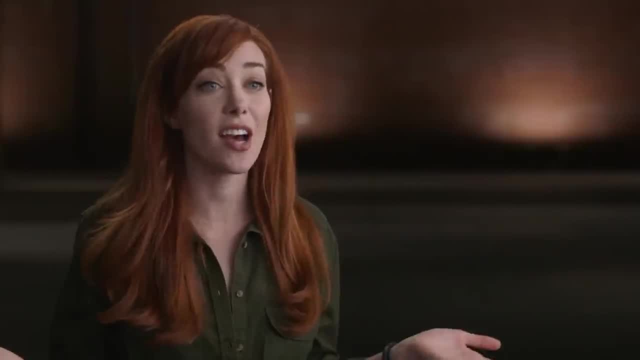 structure. but there's still the matter of that 86 000 square foot hole to cover step three. install your massive retractable roof. the university of phoenix in glendale arizona. it gets hot there. they can put a roof on and turn the ac on. ugh. only weak teams need a stadium cover. 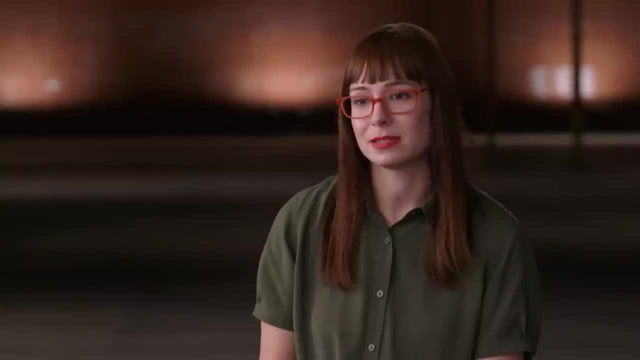 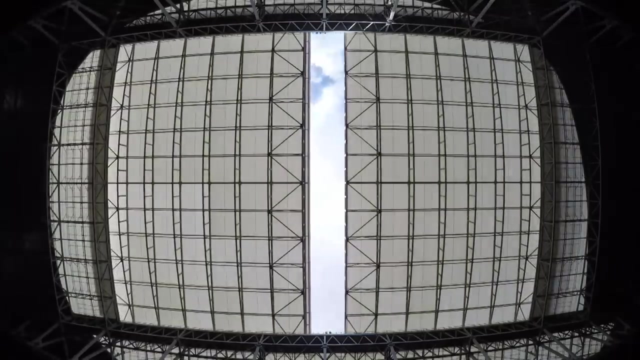 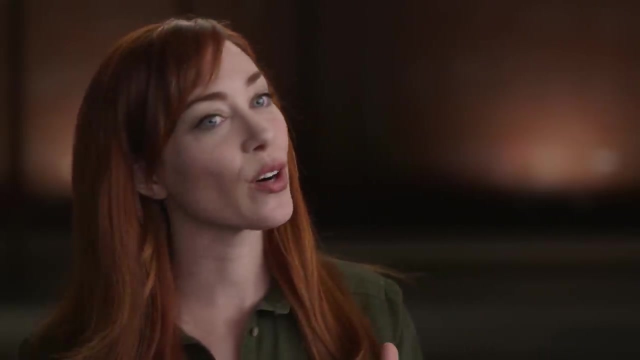 we don't have that a giant stadium. we don't need it. we welcome the elements. it makes us tougher to provide protection from sun and rain. cover your roof panels with a woven fiberglass fabric coated in teflon, called ptfe, and it stands for polytetrafluoroethylene- polytetrafluoroethylene. 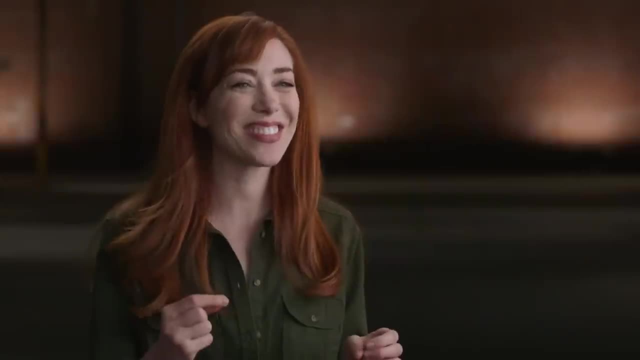 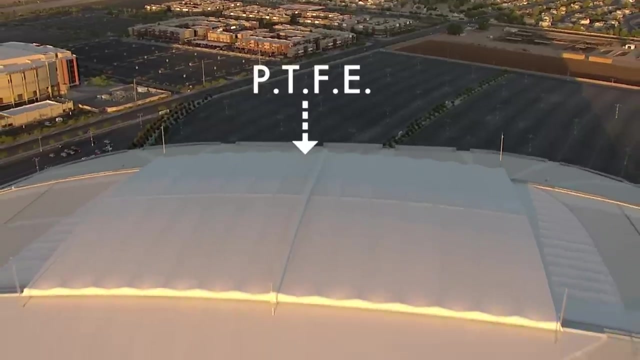 phthalene polytetrafluoroethylene. i could never say that word, just take it one syllable at a time. ptfe is a great material because it's very lightweight and it's very durable. when it that still allows some sunlight to come through. 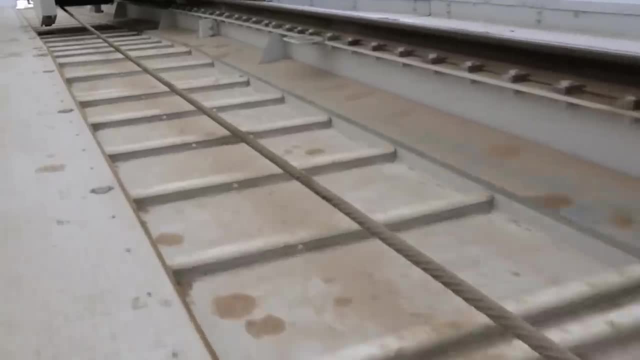 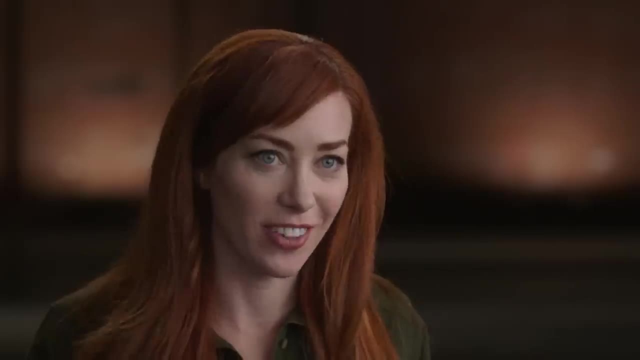 Next, install a mechanism to move the roof back and forth. So these roof panels are obviously massive. You need a lot of power to move them. This is a 2.2 million pound roof. It's a lot of pounds. So we have 64 7.5 horsepower motors. 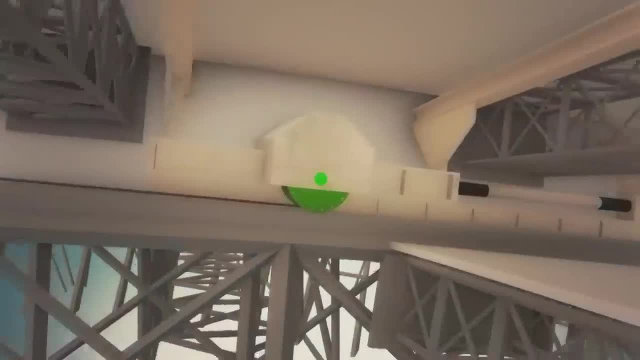 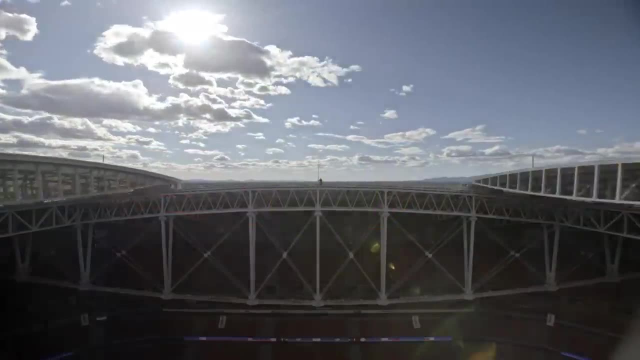 that drive 16 cable drums. These cable drums are very powerful. Each of them provides 45,000 pounds of force that move those roof panels at a quarter of a mile per hour. So it takes 12 minutes to completely open or close those roof panels. 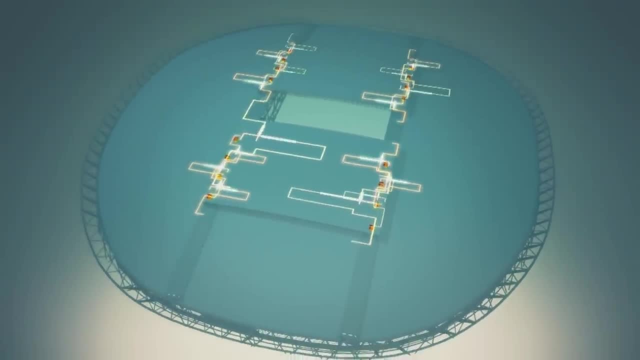 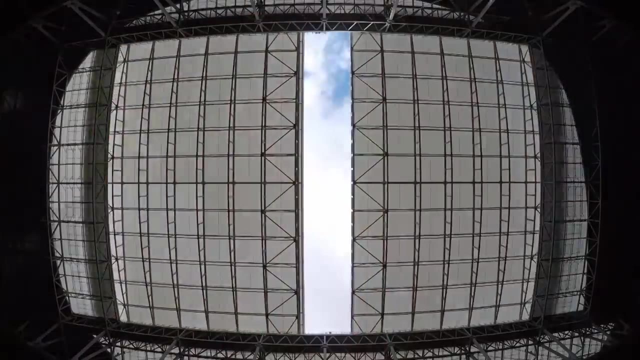 All these cable drums are synchronized with fiber optic cables to communicate with each other and make sure there's always even tension across all parts of the roof panels. Don't start getting freaky anxiety about how many millions of pounds of roof are overhead. Just don't worry. 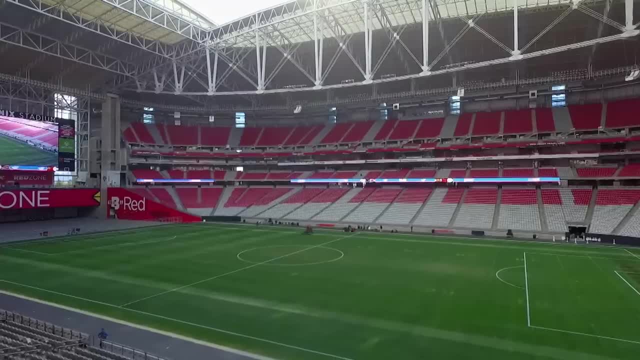 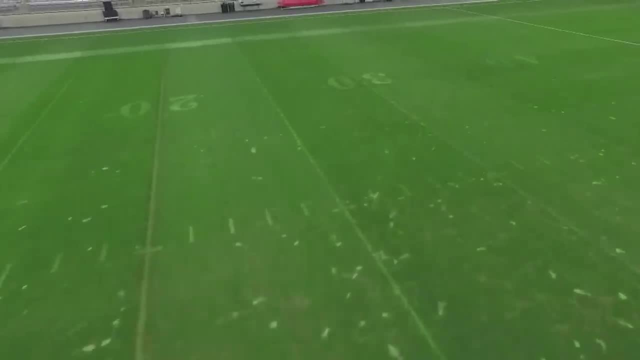 Engineers took care of it. It's fine, They got it, They worked it out. You have built yourself a first class sports stadium with a retractable roof, but the roof doesn't let in enough sunlight for a real grass playing field. Oh that grass. 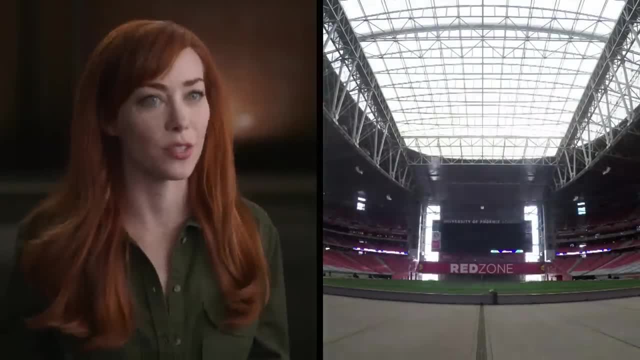 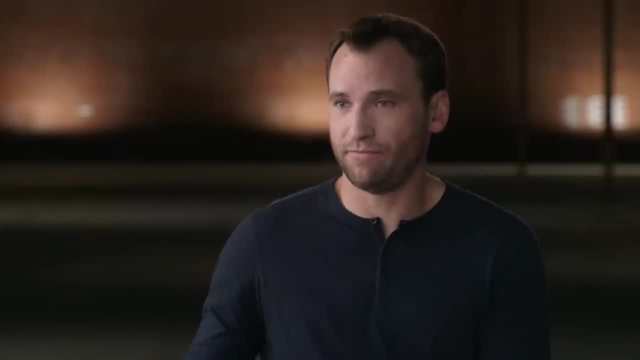 Yeah, we can retract that and keep it outside to grow when we're not using it. Step four: build a way to slide the entire field in and out of your stadium. There are two great reasons to have a movable field. One is that you can get that field outside of the stadium. 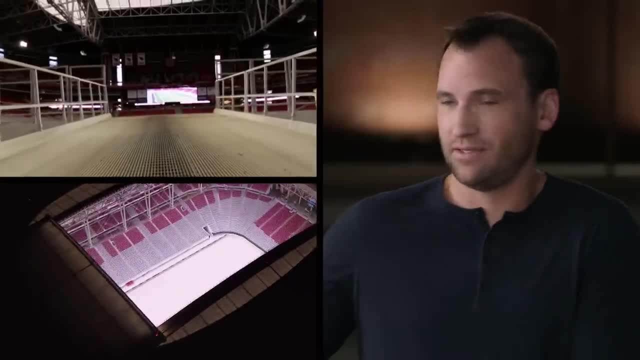 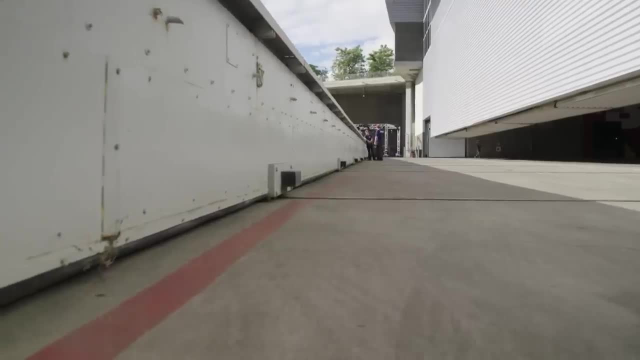 to give it direct sunlight and maintain it easier. And then you also have this empty stadium you can now use for whatever other events you want to put on without worrying about damaging this pristine field. Install 13 rails, 1,146 feet long, to move your playing field entirely out of your stadium. 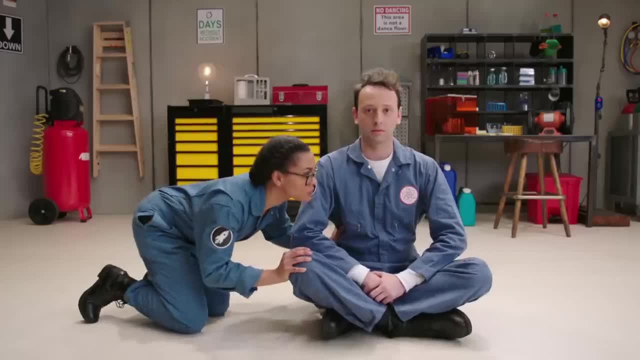 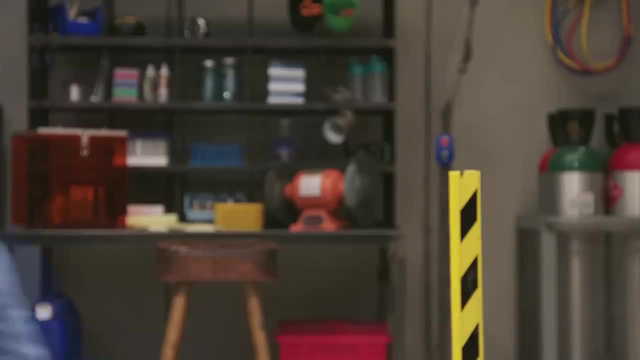 With a field that heavy sliding it's going to be no easy feat. You've got to find a way to reduce friction, to get it out of the stadium, To help move that field. it sits on 542 wheels that are each 15 inches in diameter. 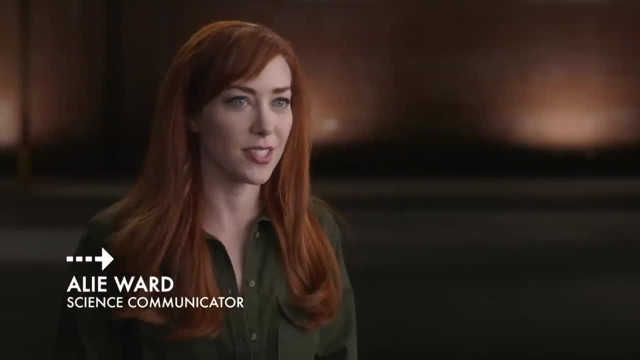 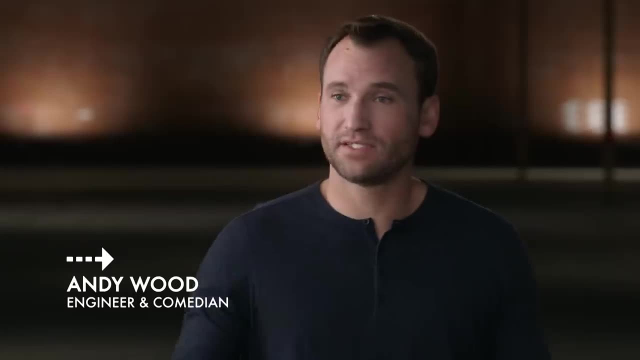 Drop that knowledge next time you go to a football game, especially if you don't know much about sports and you need something else to talk about. Step five: install your real grass playing field. The field sits in a giant tray, sort of like the world's. 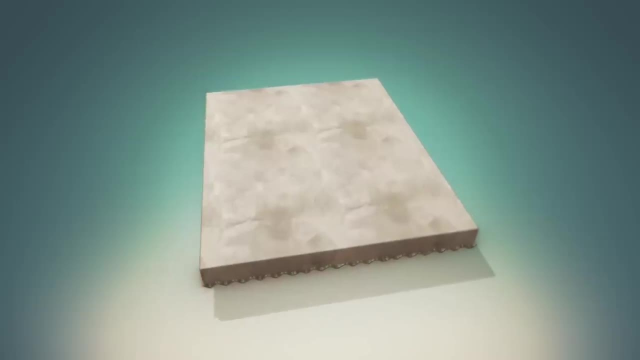 biggest lasagna. The bottom layer is corrugated steel. On top of that there's concrete and a plastic drainage mat. Over that there's 10 inches of dirt and sand And then the very top two inches of grass. 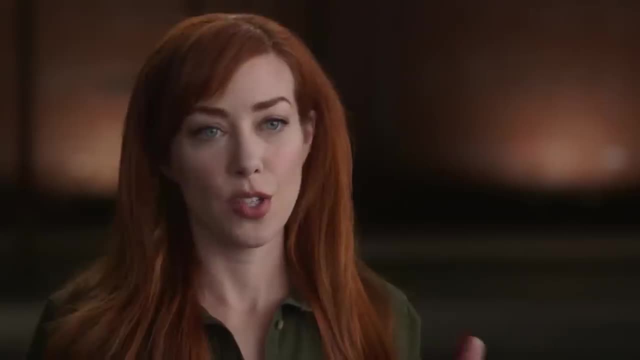 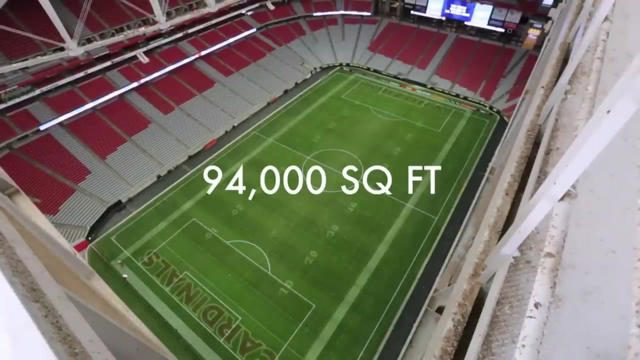 Along with all that, there are also built-in drainage and sprinkler systems. So what happens to the drainage and the sprinklers? They just kind of go with it. Sprinklers will travel With all layers in place, your 94,000 square foot playing field.